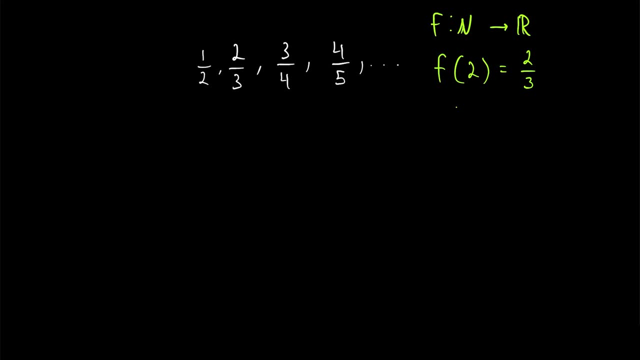 usually use traditional function notation. Instead we would write that f sub two is equal to two-thirds, and that's how we would represent the second term in the sequence f. You might notice that this sequence follows a pretty simple pattern. The fourth term, for example, has four in the numerator and the denominator is one greater, It's five. 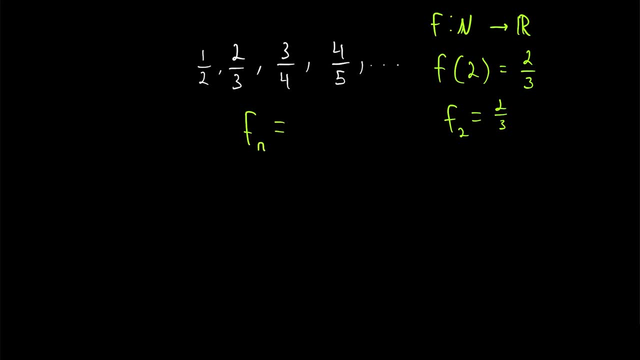 And in general for this sequence, the nth term fn is equal to n divided by n plus one. Again, looking at our example, f sub two. the second term is two divided by two plus one divided by three. 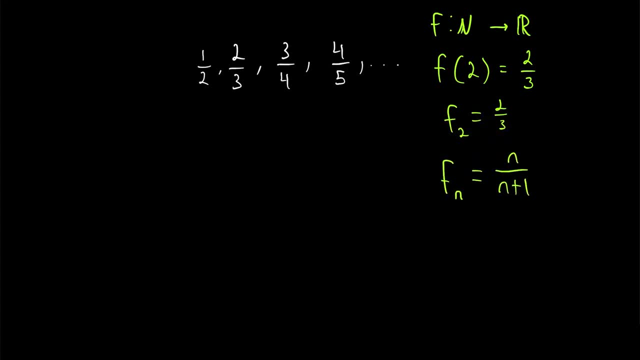 Not all sequences have this property that any term in the sequence can be easily calculated by some formula. but a lot of the sequences we'll study do, and it's quite handy If we want the 100th term in the sequence, for example, f100, that's just equal to 100 divided by 101.. 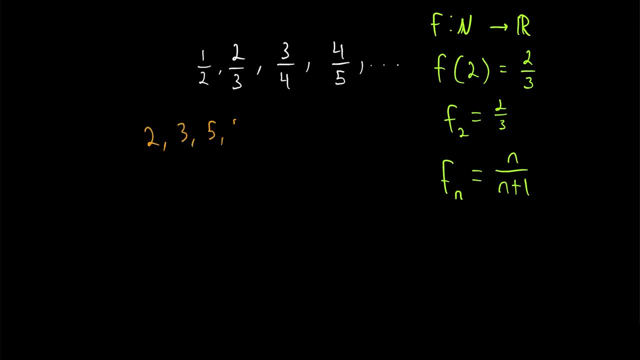 Here's an example of a sequence that cannot be described with such a simple equation: The sequence of prime numbers. We don't have a closed-form formula to calculate the nth prime number. Here's another popular example of a sequence that does have a formula for the nth term of the sequence, but it's a little. 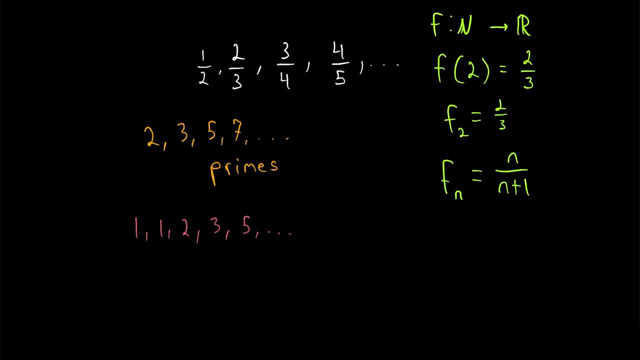 more complicated than this. This is the Fibonacci sequence, so we'll call it big F. For this sequence, the first term is equal to 1, and the second term is equal to 1 as well. But every other term in the sequence is equal to the sum of the previous two terms. So for all n greater than 2,. 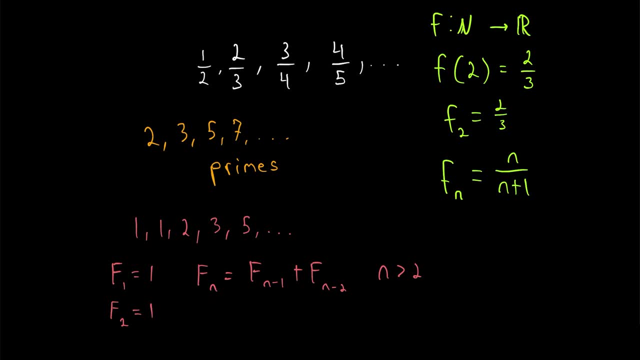 for all terms after the second term. Fn is equal to Fn-1, the previous term, plus Fn-2, the previous previous term. For example, 5 is equal to 2 plus 3.. Now let's talk a bit more. 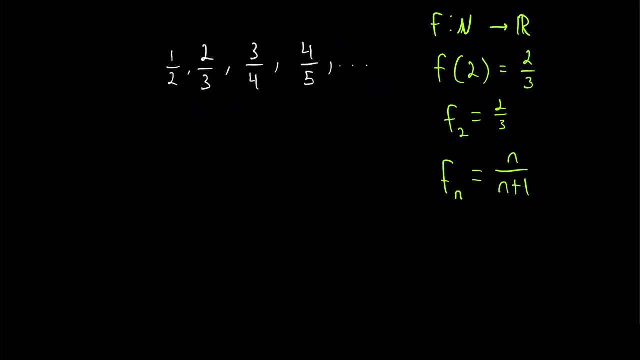 about notation. Even though sequences are ordered, unlike sets, they'll often be placed inside brackets, like we use for sets. Then, of course, we'd have to rely on context to know that this is a sequence and not a set, But one way we can make it a little more clear that it is a sequence. 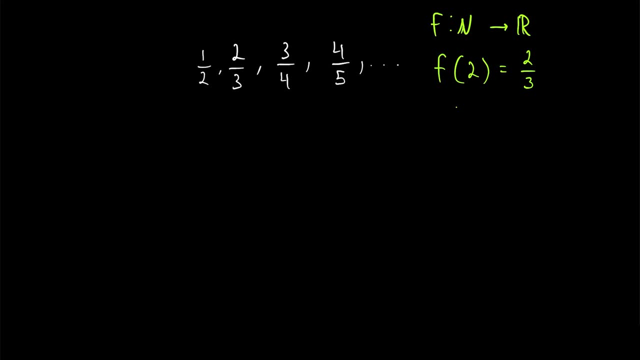 usually use traditional function notation. Instead we would write that f sub two is equal to two-thirds, and that's how we would represent the second term in the sequence f. You might notice that this sequence follows a pretty simple pattern. The fourth term, for example, has four in the numerator and the denominator is one greater, It's five. 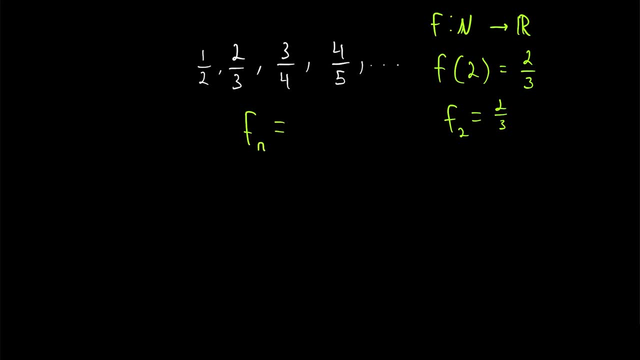 And in general for this sequence, the nth term fn is equal to n divided by n plus one. Again, looking at our example, f sub two. the second term is two divided by two plus one divided by three. 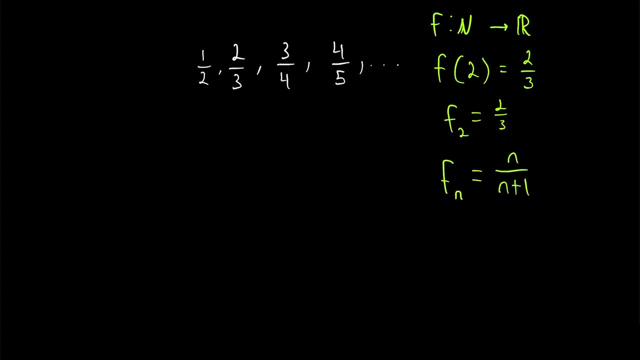 Not all sequences have this. any term in the sequence can be easily calculated by some formula, but a lot of the sequences will study do And it's quite handy If we want the one-hundredth term in the sequence, for example. 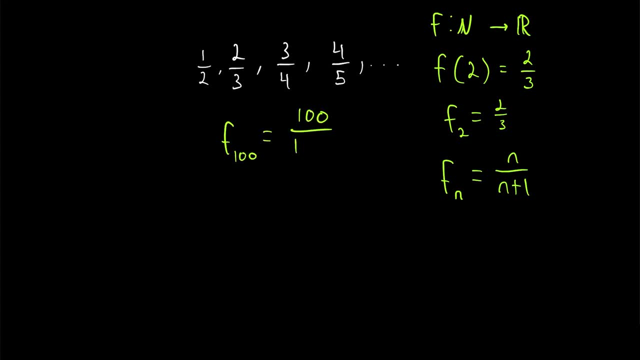 f one-hundred, that's just equal to one-hundred divided by one-hundred-one. Here's an example of a sequence that cannot be described with such a simple equation: the sequence of prime numbers. We don't have a closed-form formula to calculate the nth prime number. Here's another popular 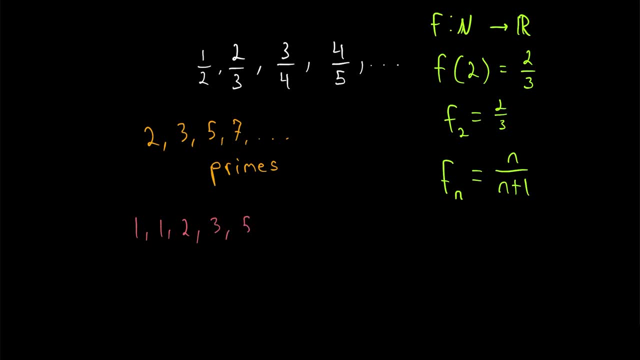 example of a sequence that does have a formula for the nth term of the sequence, but it's a little more complicated than this. This is the Fibonacci sequence, so we'll call it big F. For this sequence, the first term is equal to 1, and the second term is equal to 1 as well, But every other 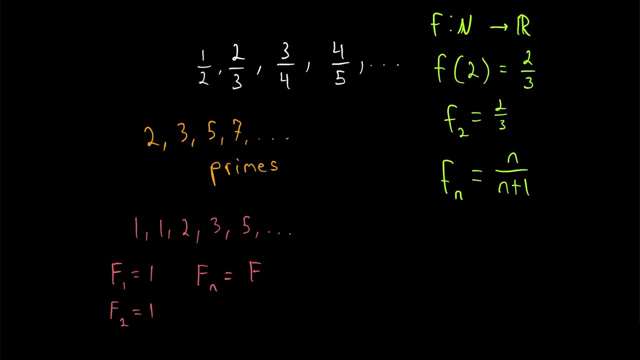 term in the sequence is equal to the sum of the previous two terms. So for all n greater than 2, for all terms after the second term, Fn is equal to Fn-1, the previous term plus Fn-2, the previous previous term. For example, 5 is equal to 2 plus 3.. Now let's talk a bit more. 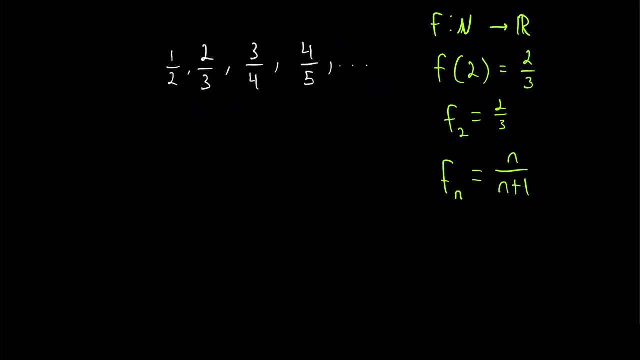 about notation. Even though sequences are ordered, unlike sets, they'll often be placed inside brackets, like we use for sets. Then, of course, we'd have to rely on context to know that this is a sequence and not a set, But one way we can make it a little more clear that it is a sequence. 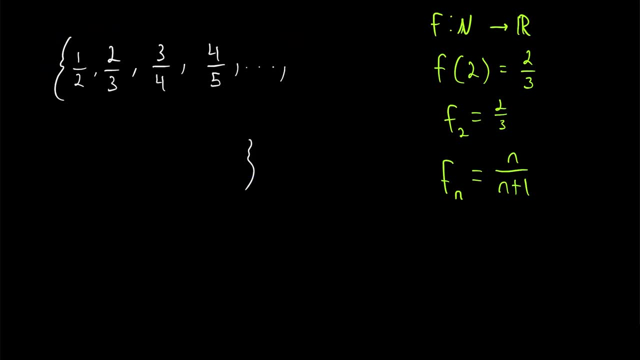 is by doing this. After the ellipses, we can write the formula for the nth term of the sequence and then put some more ellipses to indicate that the sequence continues. By doing this, we show. here are the first few terms of the sequence, for your convenience, and in general, the nth term of: 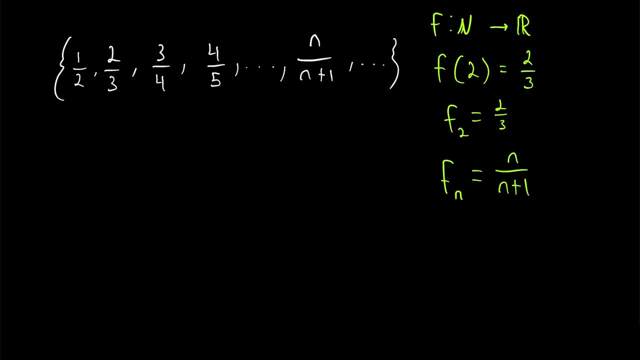 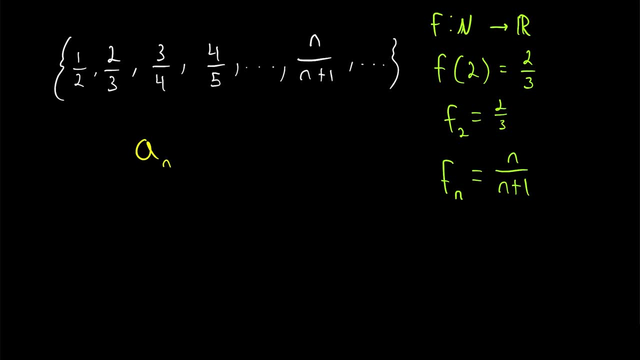 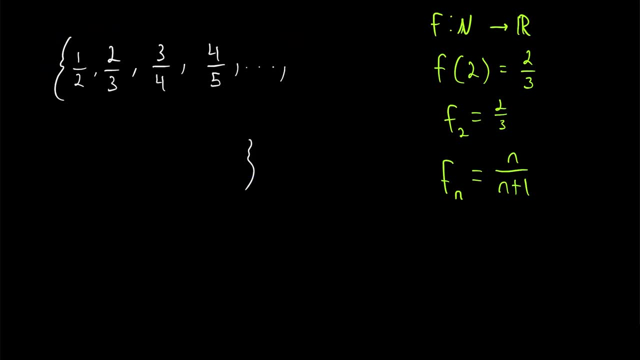 is by doing this. After the ellipses, we can write the formula for the nth term of the sequence and then put some more ellipses to indicate that the sequence continues. By doing this, we show. here are the first few terms of the sequence, for your convenience, and in general, the nth term of: 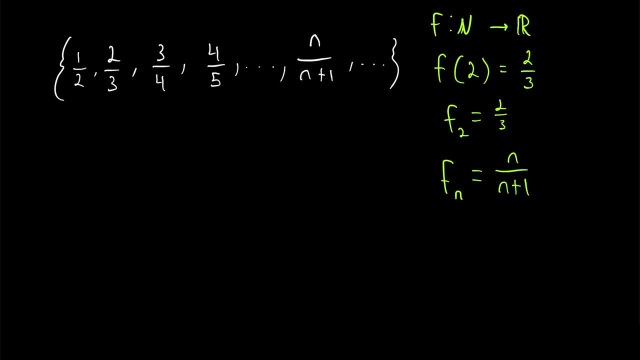 the sequence is given by this expression. Another easy way to represent a sequence, if it has a nice expression like this, is to write the formula for the nth term of the sequence and then put some more ellipses like this: for the nth term of the sequence is to give: 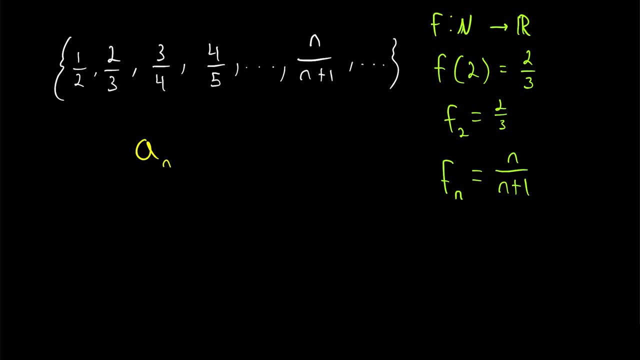 it a name like A, for example, and then just write the formula for the nth term of this sequence, So we could write that AN is equal to 1 over n. just for an example of a sequence. If we just write this, this is describing the sequence 1 over 1, 1 over 2, 1 over 3,. 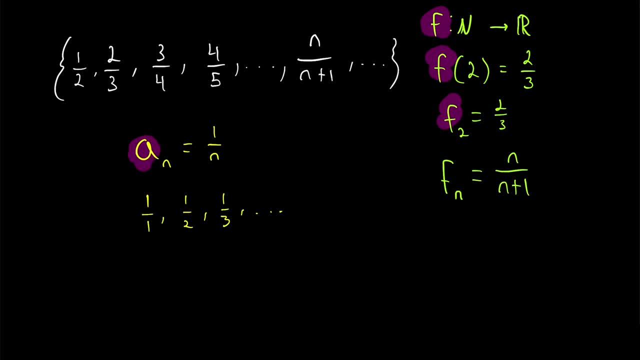 and so on. As you see, here we'll usually represent sequences with lowercase letters and a common choice: a. There is some potential for weakness in both of these notations. Neither of them explicitly say that n has to start at 1.. In this notation it's kind of implied just because we wrote the general. 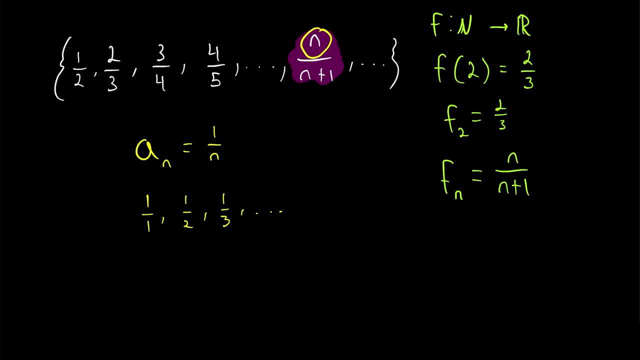 expression. and so since n is in the numerator and we see the numerator of our first term is 1, it's clear that n starts at 1.. But if we got rid of that and just wrote the sequence like this, how do we know? the sequence isn't supposed to be described by this expression: n minus 1 divided. 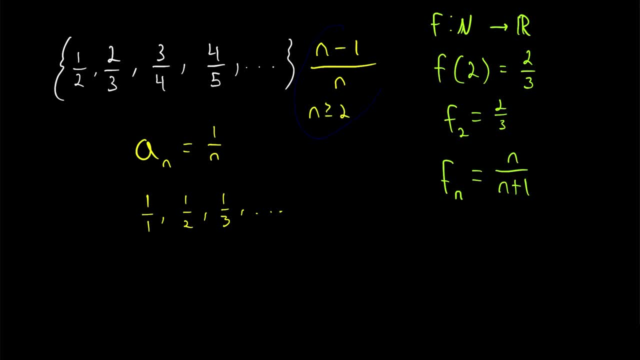 by n where n starts at 2?? Admittedly, for this sequence it doesn't make a whole lot of difference, But if, for convenience or some other reason, we want the first input value of our sequence to be 2 or 3 or something other than 1, we can do that. Just to see an example of that, as well as an. 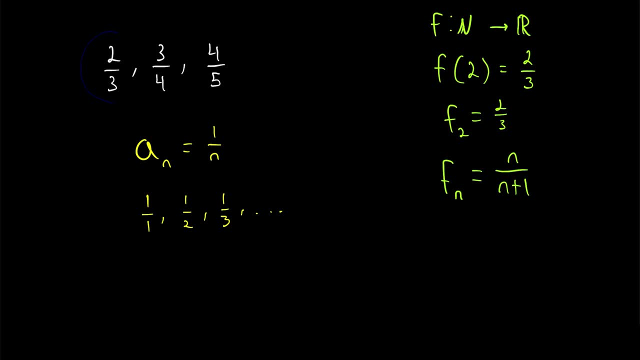 example of a finite sequence. let's modify the sequence in white, So we're just looking at this sequence of three terms. Then we can still think of it as a function, but its domain is no longer the natural numbers. Instead, we could represent this sequence as the function with a. 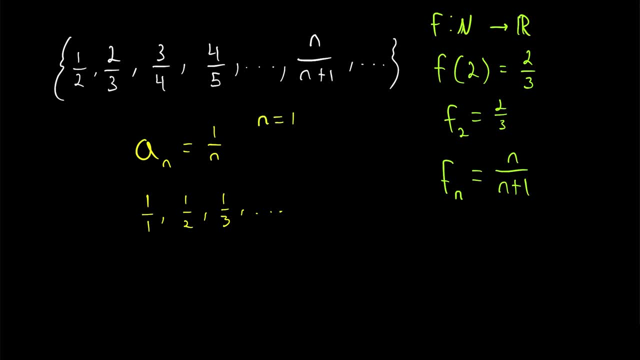 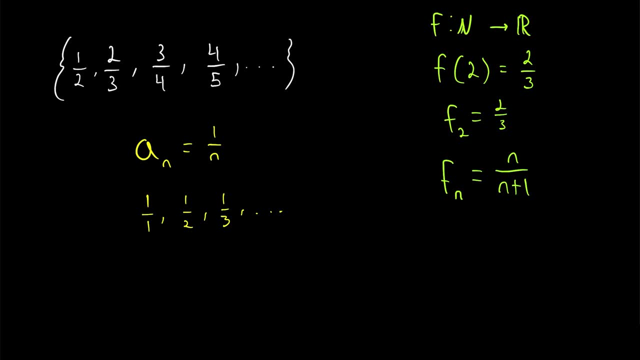 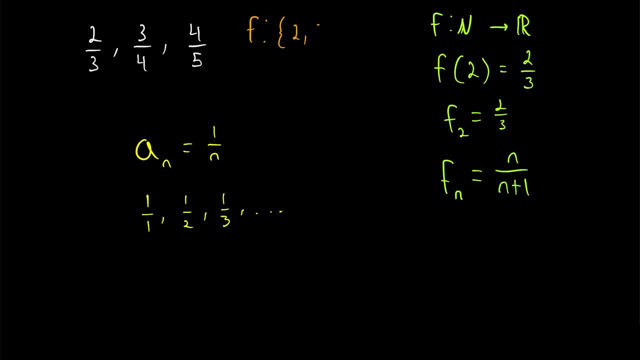 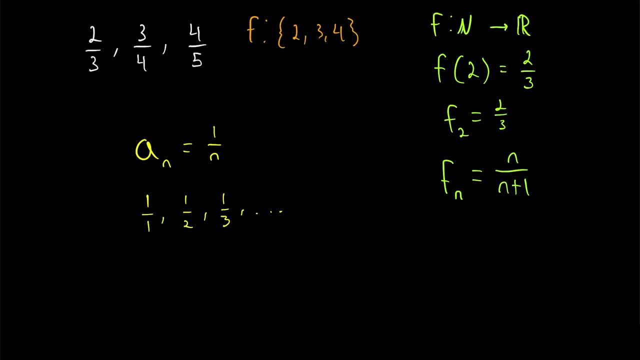 domain of the set containing 2,, 3, and 4, and its codomain is just the real numbers And the function, just as before, is defined by n over n plus 1.. So then if we plug in 2, we would get 2 divided by. 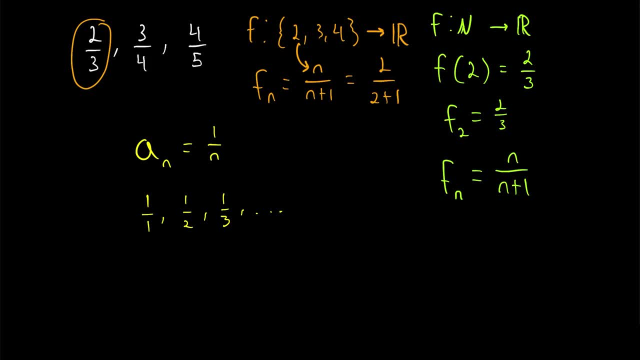 2 plus 1, which is 2 over 3. The first term of our sequence. So that works just fine. However, I think it's clear why it might be preferable for n to start at 1.. For example, with this sequence, if we write f sub 2: 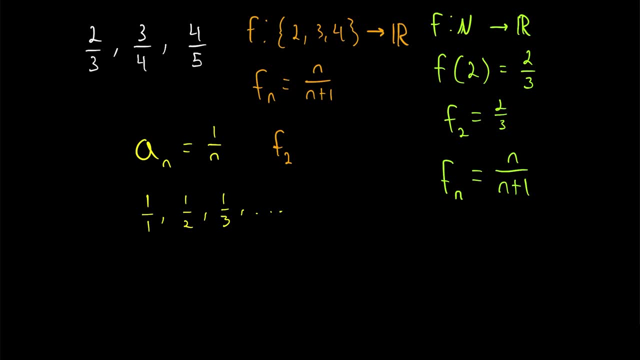 and we're not being super clear. it might be kind of confusing. Is this supposed to mean the function describing the sequence with an input of 2? Or is f2 supposed to refer to the second term of the sequence? Thankfully, if we want to, we can change the expression. 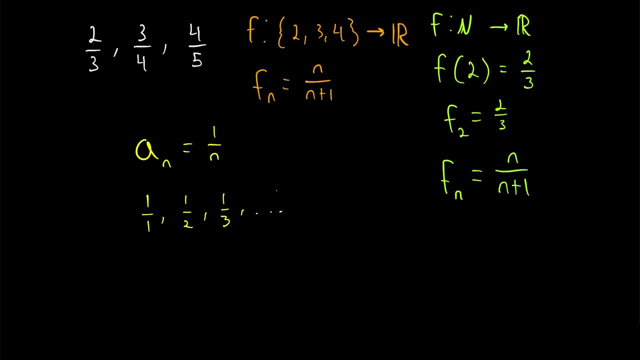 that describes our sequence, so that n can start at 1.. So for this sequence, as an example, we could rewrite the expression as n plus 1 divided by n plus 2. And then we can change our domain to what we want it to be, starting with 1, and then we also have 2 and 3.. Then the 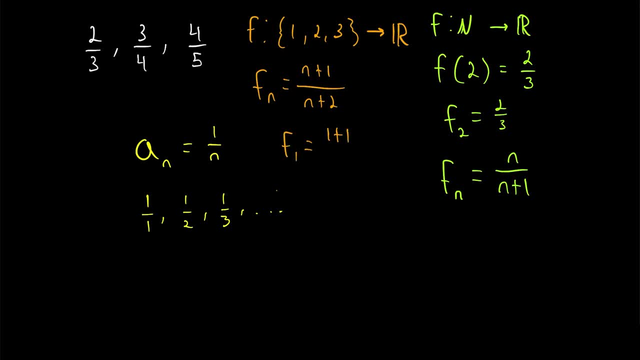 first term of the sequence, f1, is equal to 1 plus 1 divided by 1 plus 2, which is equal to two-thirds, and that is indeed the first term of the sequence. However, if we really want n to not start at 1,, there is some handy notation to represent that. 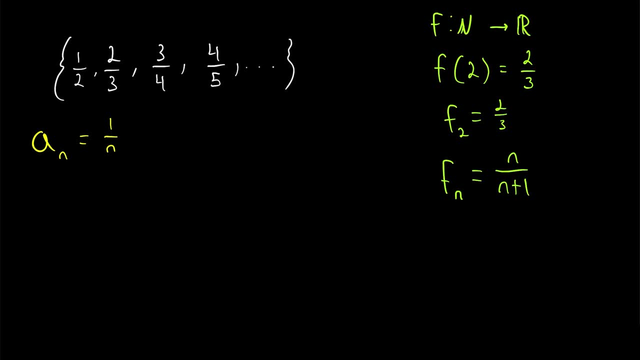 Let's continue to consider this sequence: a n equals 1 over n. Another way we could write this sequence is by using set brackets, like we did earlier, but instead of listing terms of the sequence to describe the pattern, we just describe the pattern with the expression that defines it. 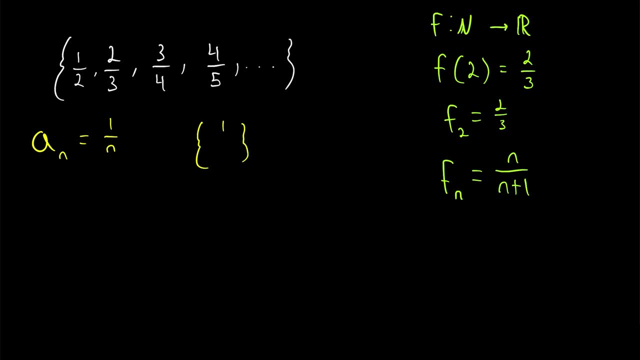 So we would write curly brackets and inside we put the expression for terms of the sequence one orient over n. And then if we want n to start at something other than 1, we can write that at the bottom. We can say n starts at 3,, for example. And if we want it to be an infinite sequence, we can write: 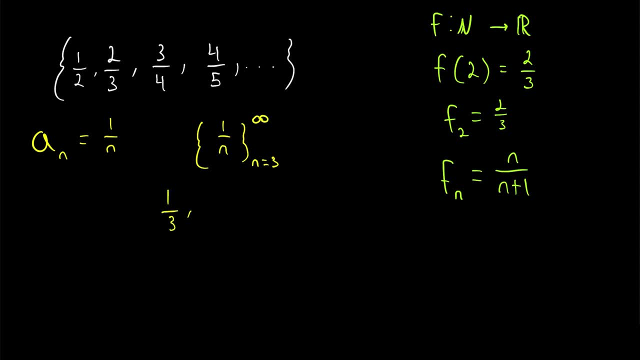 infinity at the top, And this describes the sequence 1, 3rd, 1 4th, 1 5th and so on. However, if we wanted the sequence to stop at n equals 5, we could write 5 at the top and then our sequence. 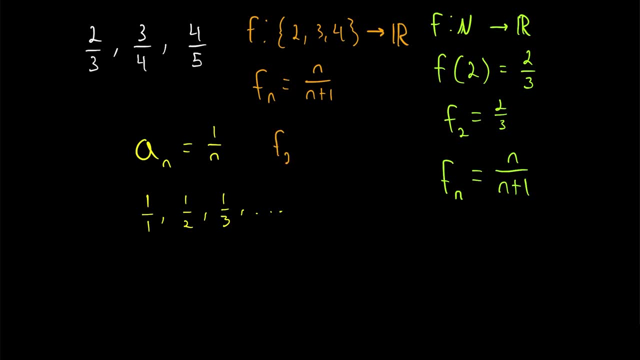 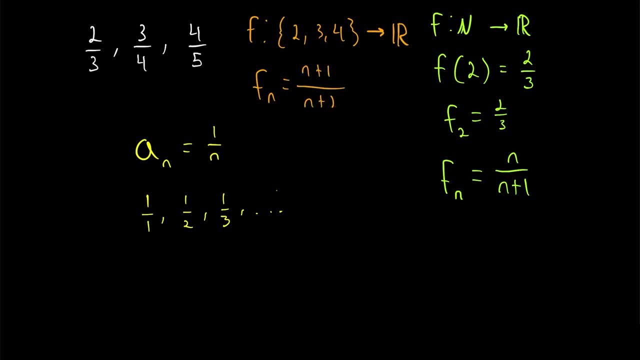 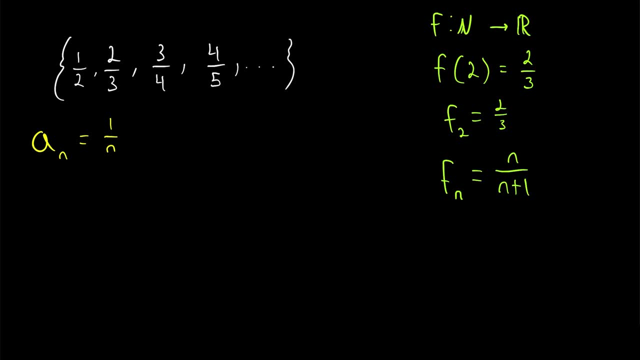 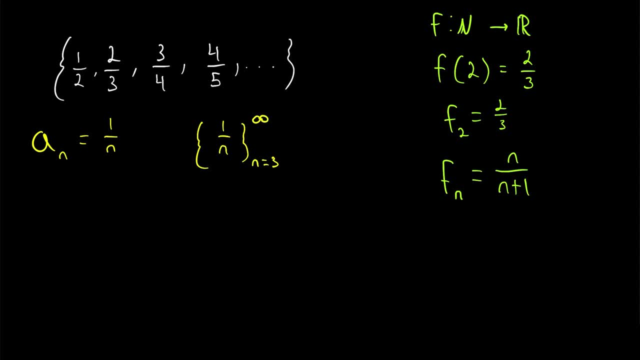 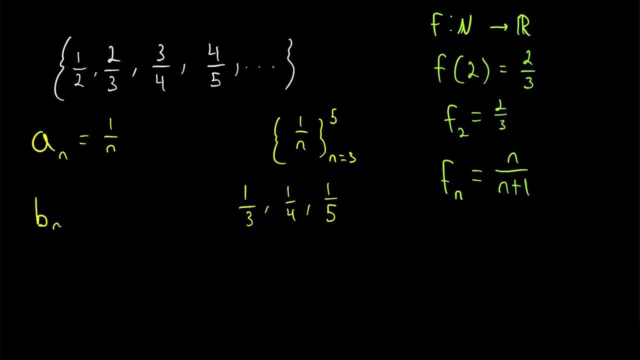 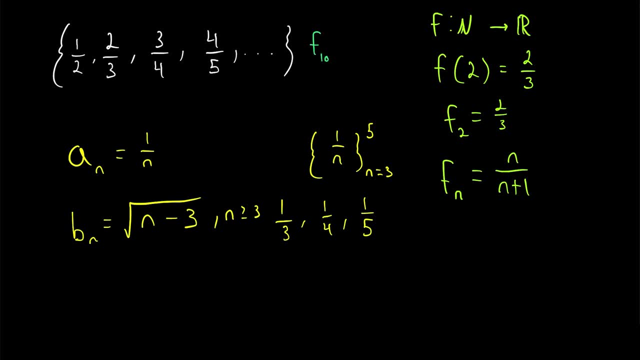 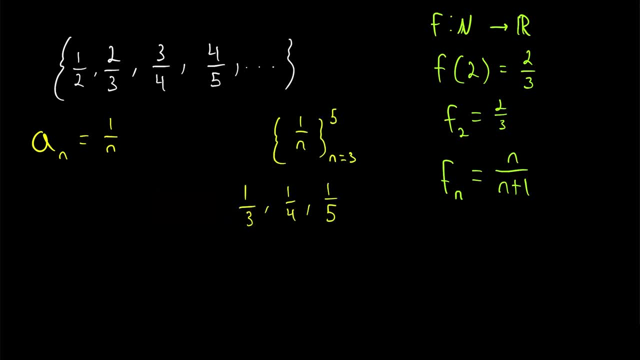 would just consist of these three terms In general. if we represent a sequence using some expression like this and we don't specify that n is greater than or equal to some value that we want it to start at, it will be assumed that n starts at 1.. Or we may also have to assume that 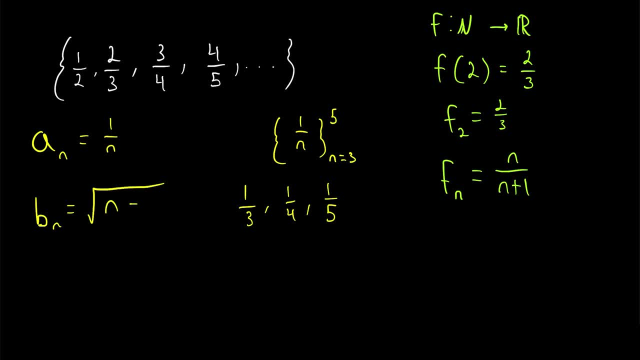 n starts at the smallest positive integer for which the expression is defined. For example, for this expression we might assume that n is greater than or equal to 3,, so that the sequence would just consist of these three terms. And if we represent a sequence using some 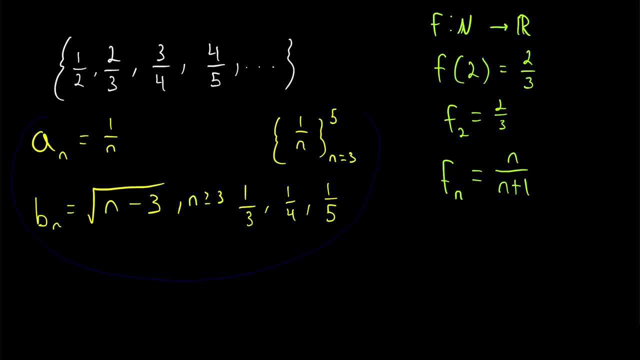 real numbers. So there's a bunch of fun notation for you. Now let's quickly touch on a little bit more vocab. Do you notice if the terms of this sequence are approaching any particular value? It looks like the terms are getting closer and closer to 1.. For example, the 100th term of the 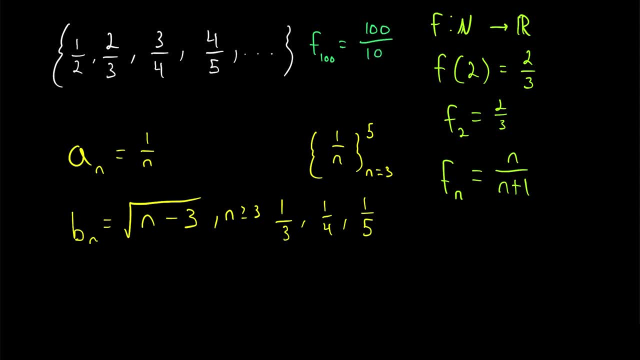 sequence which we looked at a few minutes ago is equal to 100 over 101. That's approximately 1.. Not quite, but almost. When the terms of a sequence get arbitrarily close to some value, like 1- in this case, we call that value the limit of the sequence. 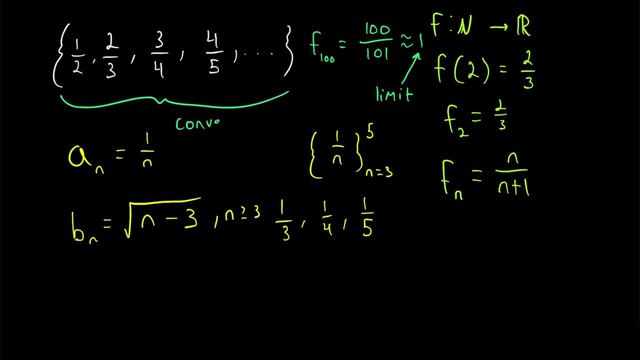 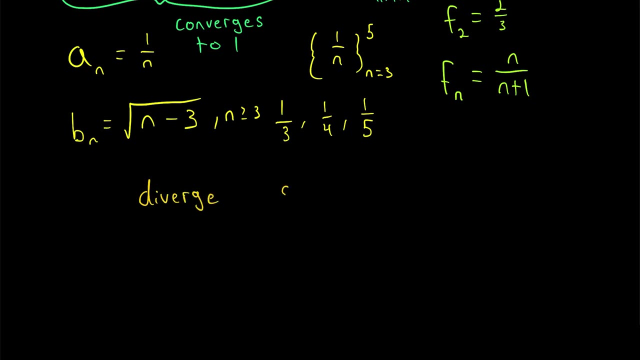 Furthermore, we say that the sequence converges to its limit. So we would say that this sequence converges to 1.. We will, of course, talk about these terms and their definitions in detail in future lessons. A sequence that doesn't converge is said to diverge, For example: 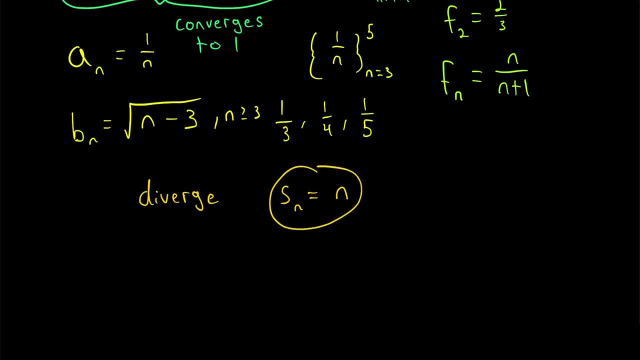 the nth term of this sequence is equal to n. This sequence diverges. Its terms get bigger and bigger. So in fact we would say that this sequence not only diverges, but it diverges to positive infinity. Some sequences diverge to negative infinity. 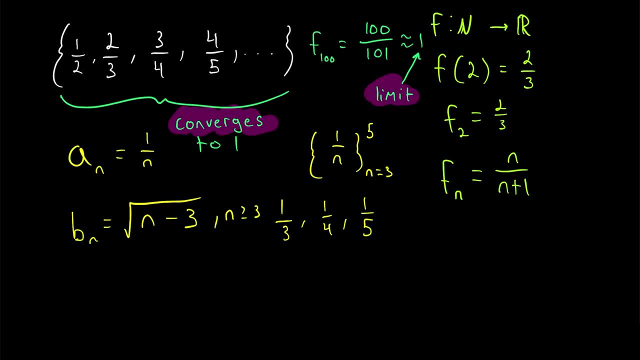 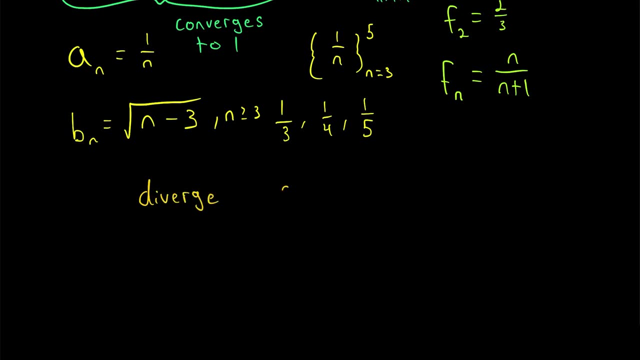 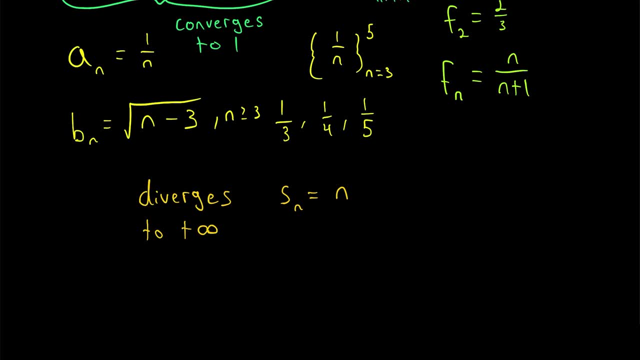 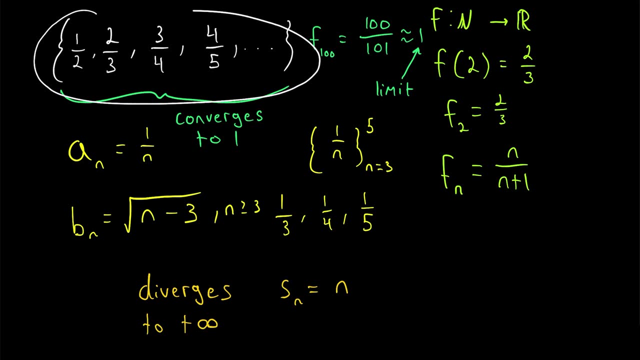 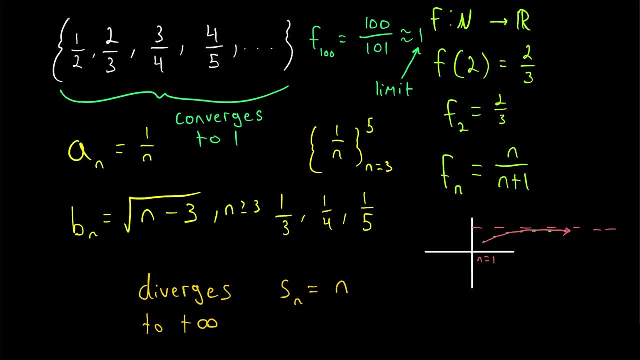 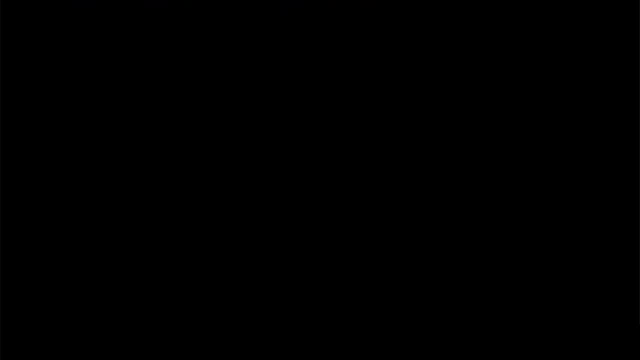 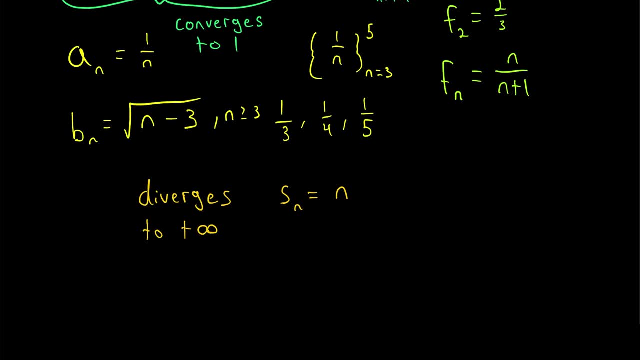 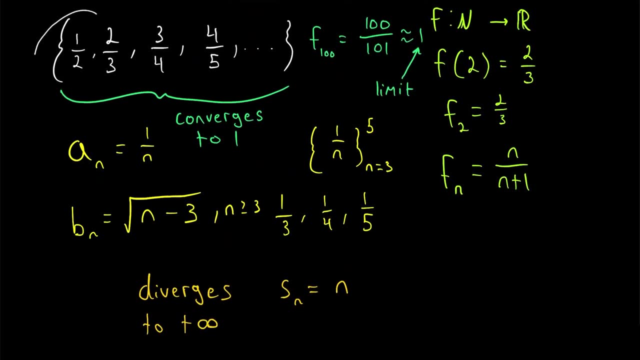 and some divergent sequences don't diverge to positive or negative infinity. We can, of course, get some idea of a sequence's behavior by plotting it on a graph. If we were to plot this sequence on a graph, for example, we'll plot it down here in the bottom right, where we've still got some room. 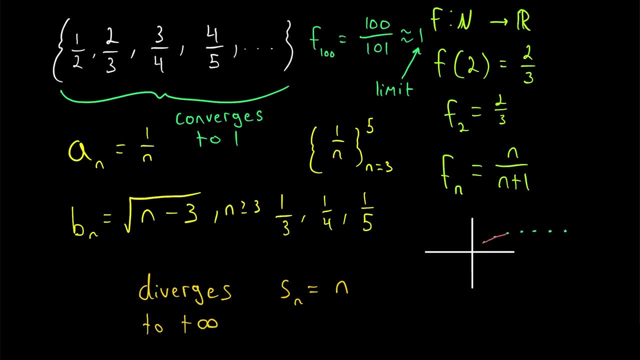 it would look something like this, And we could, of course, draw a line through the points of the sequence to get a smooth curve if we wanted to. When n equals 1,, the sequence is equal to one half, And then it gets bigger and bigger, continuing to approach a value of 1, but never. 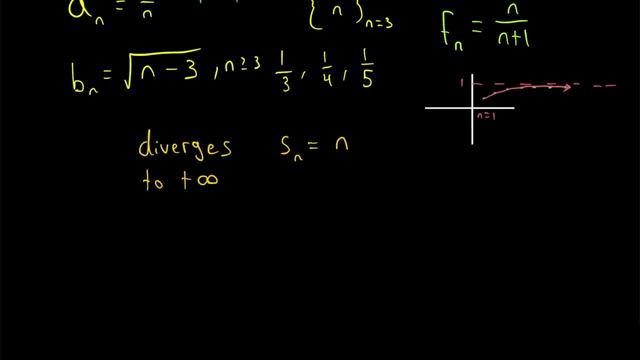 quite getting there. That's the limit. For the purpose of proofs, we may find it useful at times to represent a generic sequence. For example, we might do that by writing a sub n in brackets. Or, if we needed to, we could put our sequence in set brackets. just say sn. for another example, 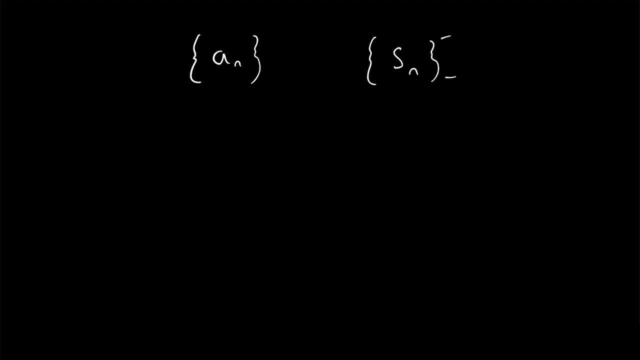 and write the starting and ending points for n on the top and bottom, like we did earlier. For example, maybe n starts at 5 and goes to positive infinity, or maybe it goes to positive 10.. One other generic way we could describe a sequence similar to the first way we wrote one. 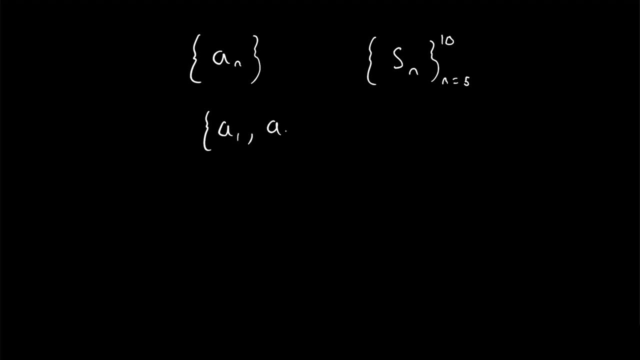 down is to list some generic terms like a1, a2, a3. And so on, in set brackets. Similar to what we did earlier, we could also, after the ellipses, put a comma and then write a general term, an, and then put some more ellipses. 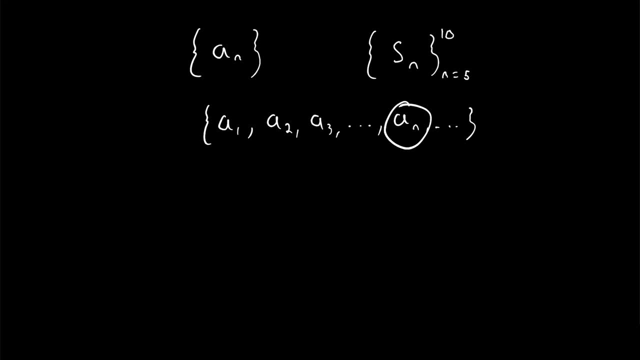 Having the an in there is nice because it lets the reader know that we're going to represent a generic term from our sequence as an. So there's a bunch of introductory material for you, some vocab and notation. For one last exercise, let's try rewriting this sequence, but in terms 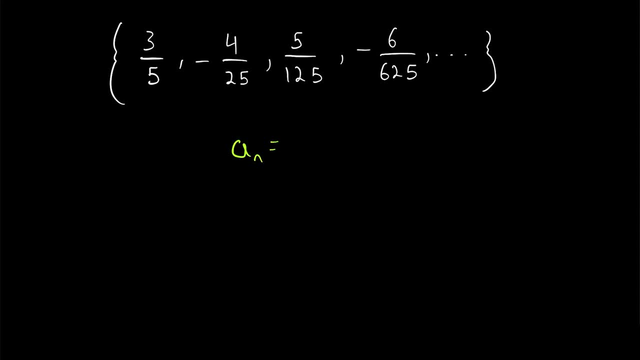 a handy expression like an is equal to something, an expression for the nth term of this sequence. Let's take a close look at the terms of the sequence. The numerators start at 3, and then go up 1 each term. Meanwhile, in the denominators, 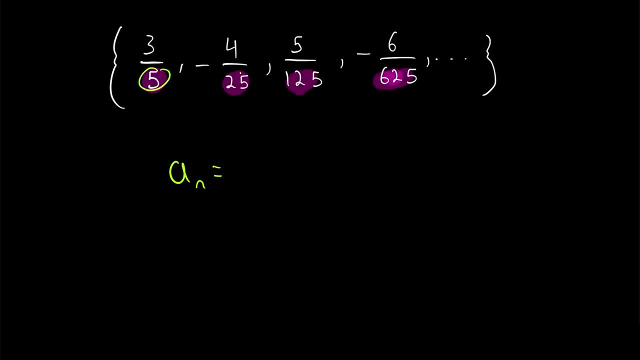 we have increasing powers of 5, 5,, 5 squared, 5 cubed, and so on. The only other detail we've got to deal with is that the signs of the terms are alternating: positive, negative andottentic. the signs of the terms are alternating positive, negative. 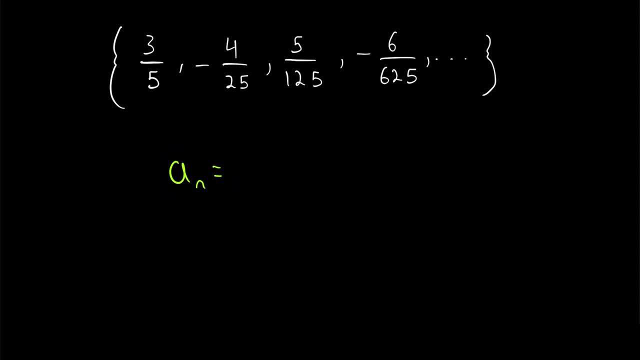 positive andottentic. The only other detail we've got to deal with is that the signs of the terms are positive- negative. So for our general expression, we might write n in the numerator and say that n has to be greater than or equal to 3.. However, since we'd rather have n start at 1,, we can just 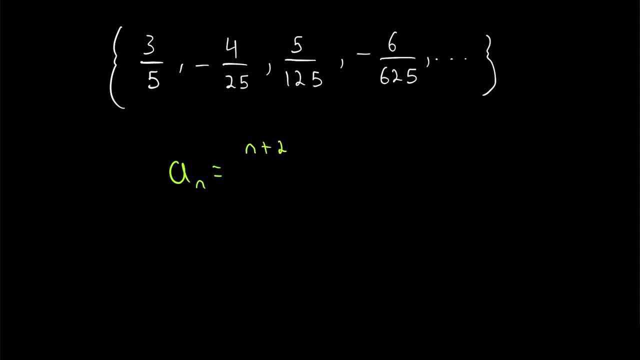 write n plus 2 in the numerator instead. Then when we plug in n equals 1, we'll get 3 in the numerator, just like we want for the first term For the denominator. we just have to divide by 5,. 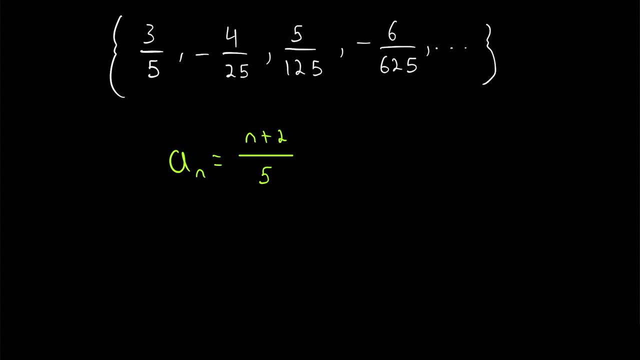 and 5 is being raised to an increasing power. So raise 5 to the power of n, Then in the first term, we'll have 5.. In the second term, we'll have 5 squared, and so on. Lastly, how are we going to? 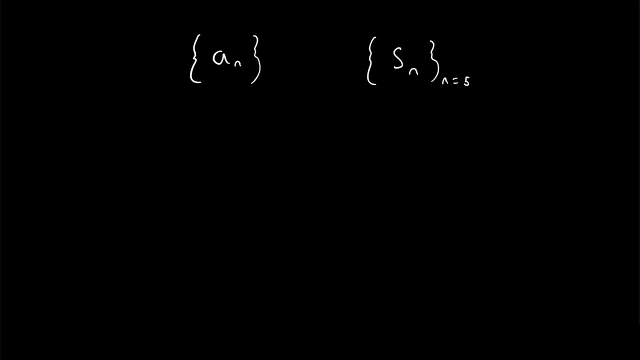 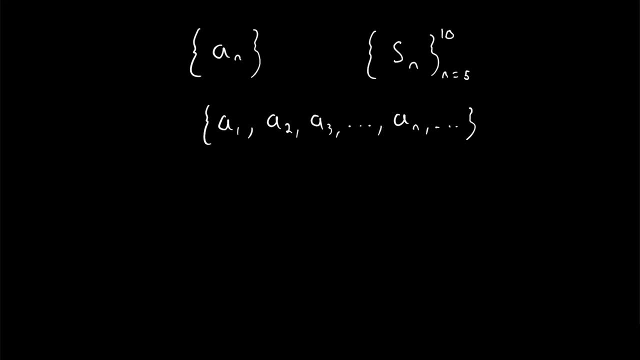 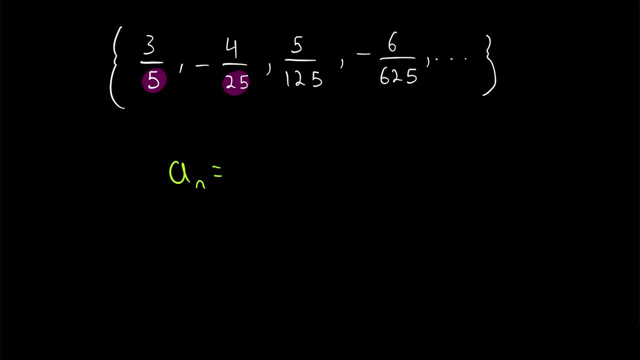 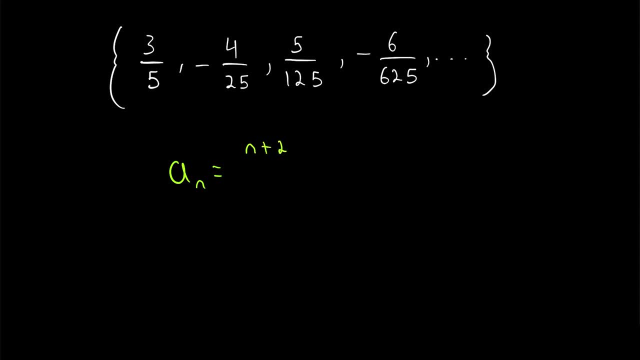 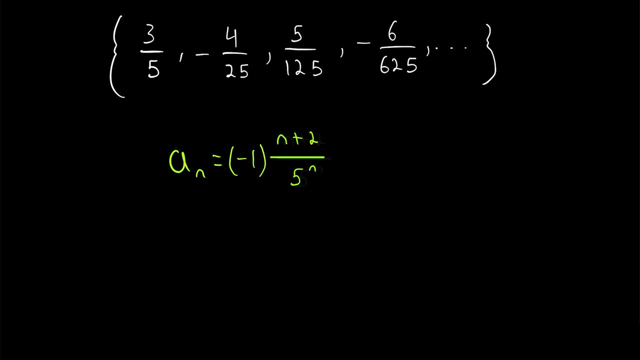 and then put some more ellipses to indicate that the sequence continues. After the ellipses, we can write the formula for the nth term of the sequence, And so we'll just have a positive first term, like we want. And there it is. that is our expression for the nth term of this sequence. 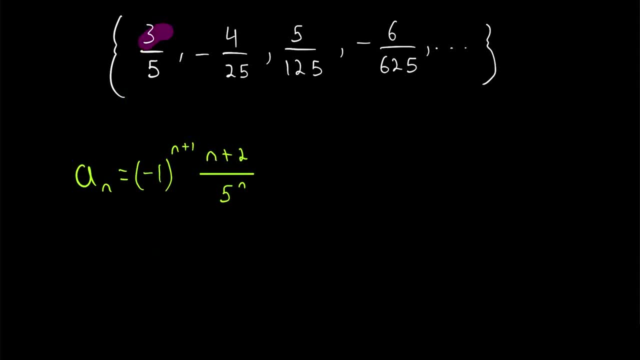 And so we'll just have a positive first term, like we want. And there it is. that is our expression for the nth term of this sequence. So we could describe the sequence like this, or we could just use this instead, which, frankly, is more useful. 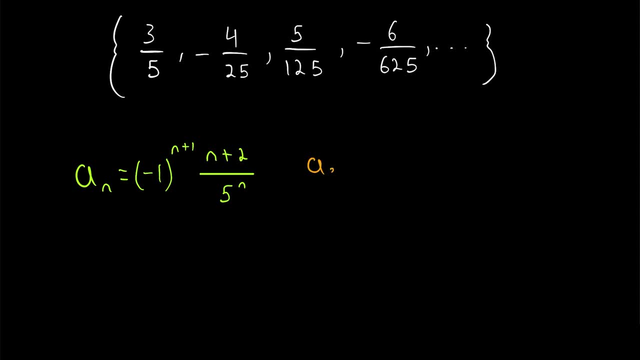 Let's just take our expression for spin and plug in. n equals 3.. The third term of the sequence, according to our expression, is negative 1 to the power of 3 plus 1, multiplied by 3 plus 2, divided by 5 to the power of 3.. Negative 1 to the power of 3 plus 1 is negative 1 to the power of 4, which is: 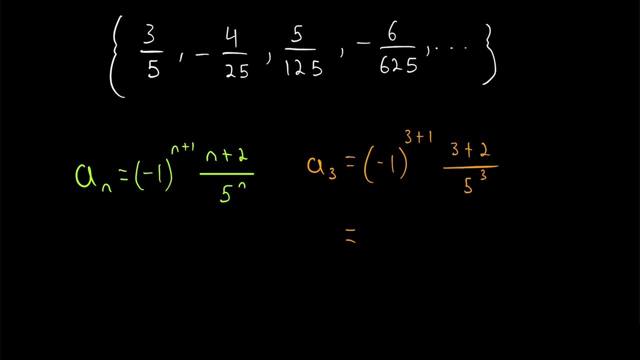 just 1.. Then 3 plus 2 is 5.. 5 to the power of 3 is 125.. And there we go. That is the third term of our sequence and we see that it is correct And I think that'll do it for today. So I hope this. 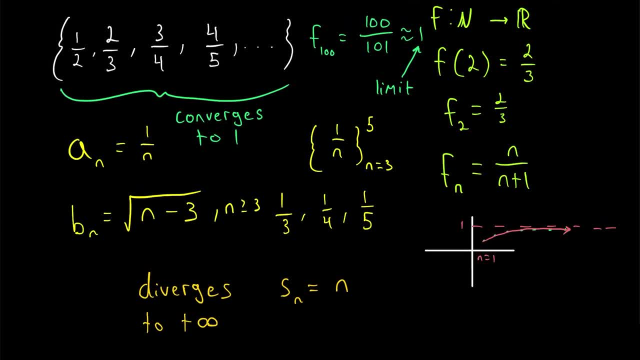 video helped you understand some language and notation that we use when talking about sequences. Let me know in the comments if you have any questions, need anything clarified or have any other video requests. If you find Wrath of Math helpful, I hope you'll consider supporting.